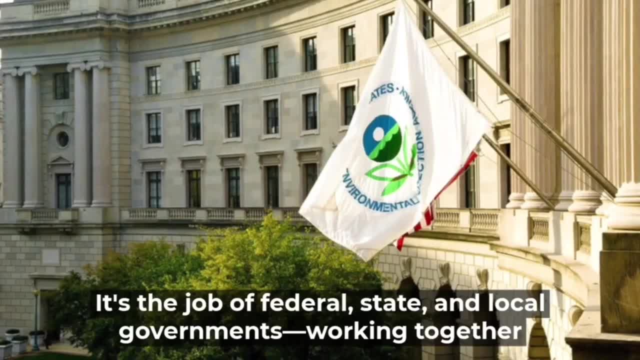 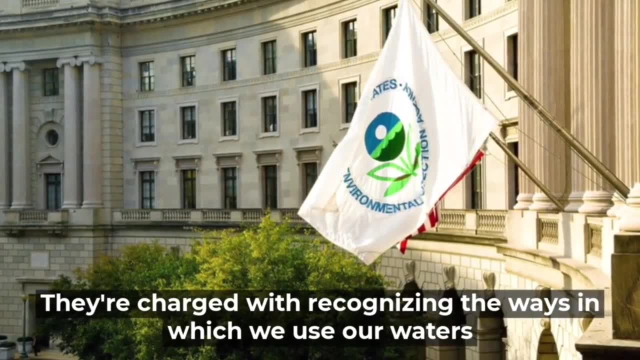 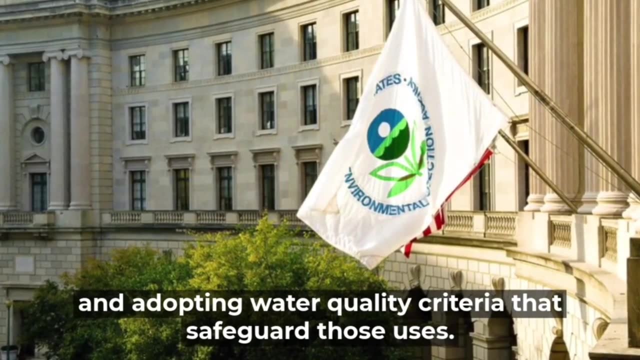 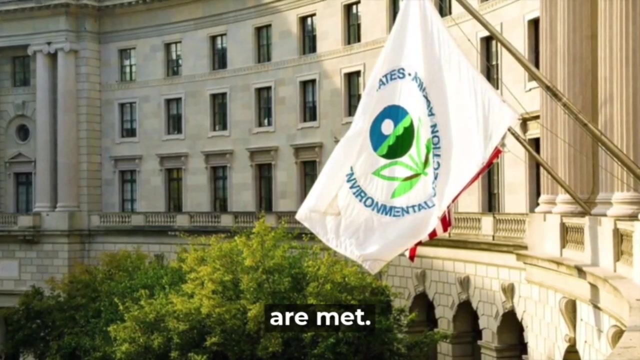 It's the job of federal, state and local governments, working together to achieve the goal of the Clean Water Act. They're charged with recognizing the ways in which we use our waters and adopting water quality criteria that safeguard those uses. They also have the responsibility to implement plans and protections to ensure water quality criteria are met. 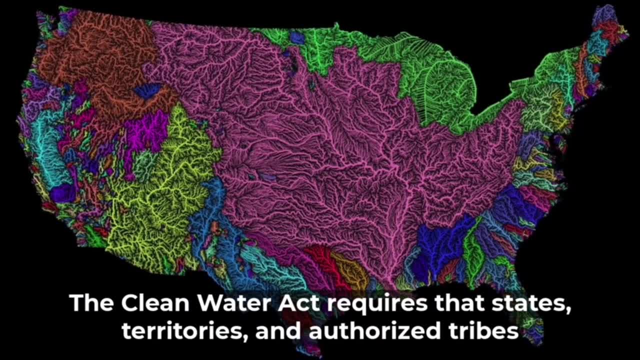 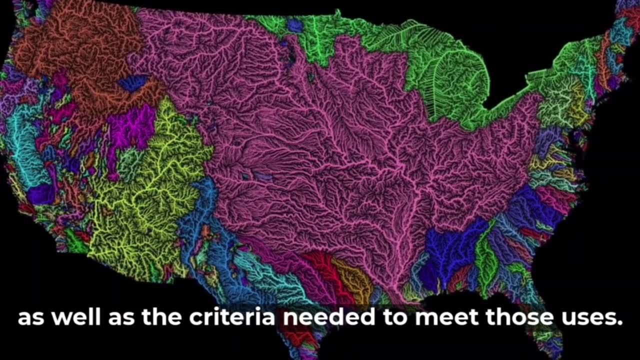 The Clean Water Act requires that states, territories and authorized tribes recognize our water's uses, as well as the criteria needed to meet those uses. The Clean Water Act requires that states, territories and authorized tribes recognize our water's uses, as well as the criteria needed to meet those uses. 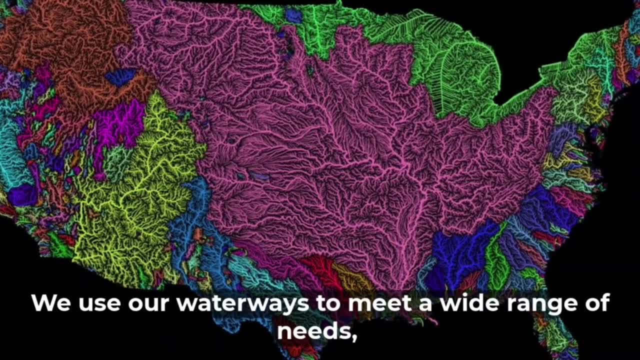 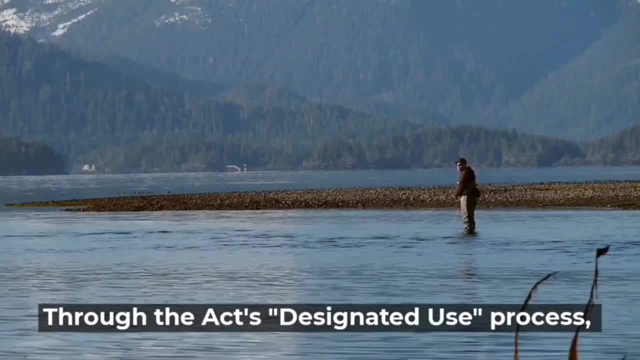 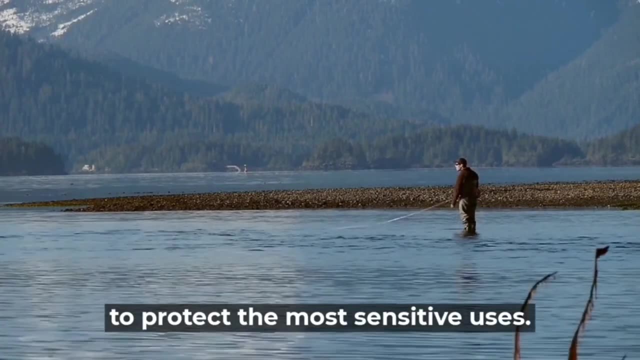 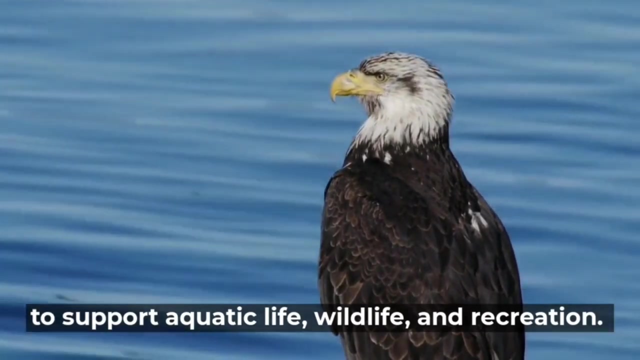 We use our waterways to meet a wide range of needs, from drinking water supply to hydroelectric power. Through the Act's designated use process, states are tasked with setting goals to protect the most sensitive uses. At minimum, they are required to designate uses for all streams to support aquatic life, wildlife and recreation. 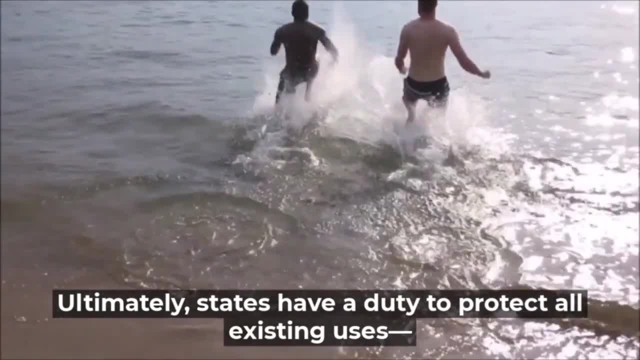 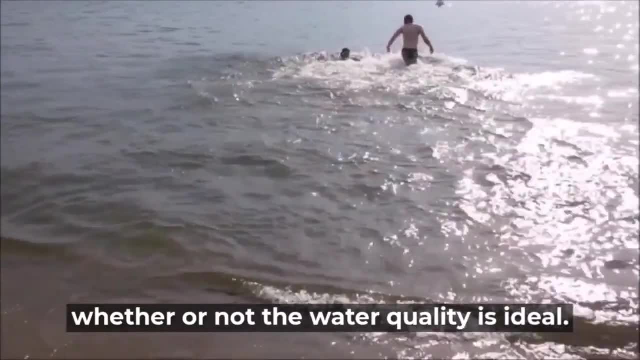 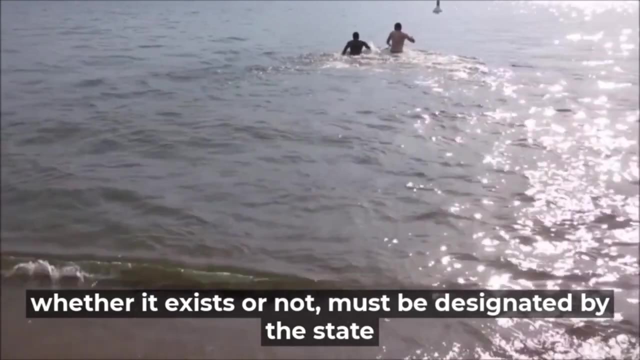 States have a duty to protect all existing uses, all the ways our communities depend on our waters, whether or not the water quality is ideal. Any use that is reasonably attainable for a particular body of water, whether it exists or not, must be designated by the state and reflected in state water quality standards. 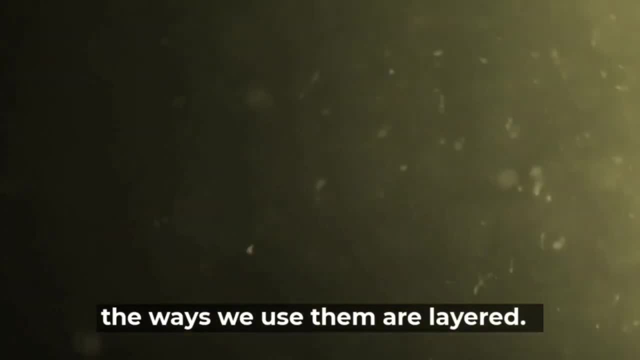 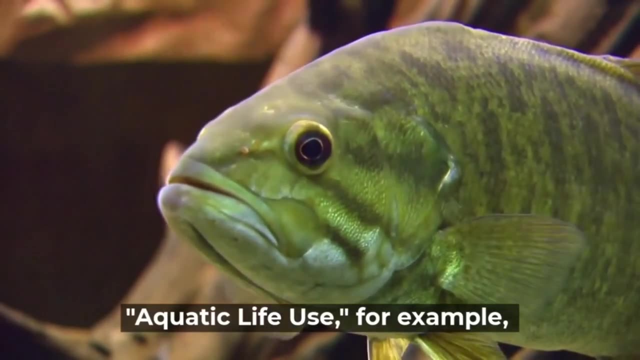 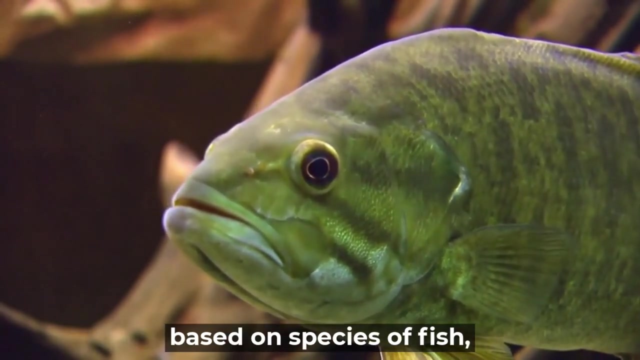 Like the waters themselves, the ways we use them are layered, and water uses can be categorized differently from state to state. Aquatic life use, for example, is one type that is broadly shared, but some states have more specific uses based on species of fish. 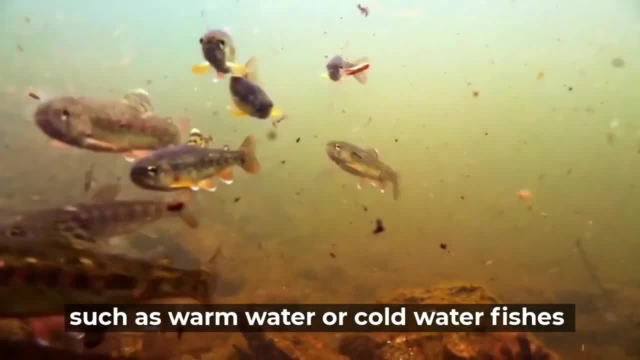 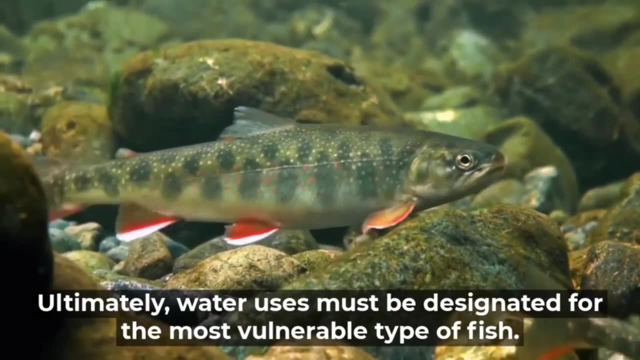 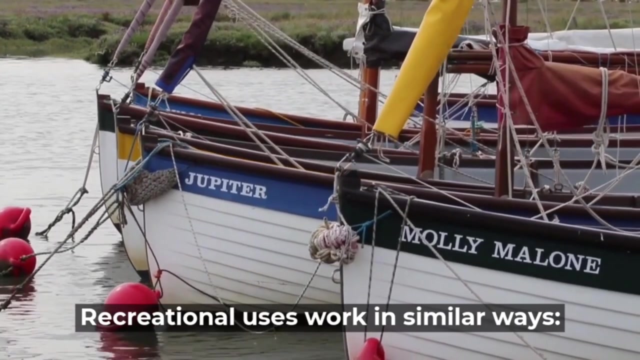 such as warm water or cold water fishes, or those that migrate versus those that are stocked. Ultimately, water uses must be designated for the most vulnerable type of fish: Recreational uses- Recreational uses- work in similar ways. Some segments of our waterways are designated for secondary contact recreation. 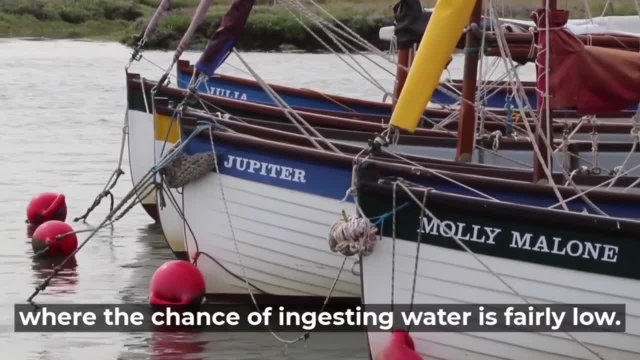 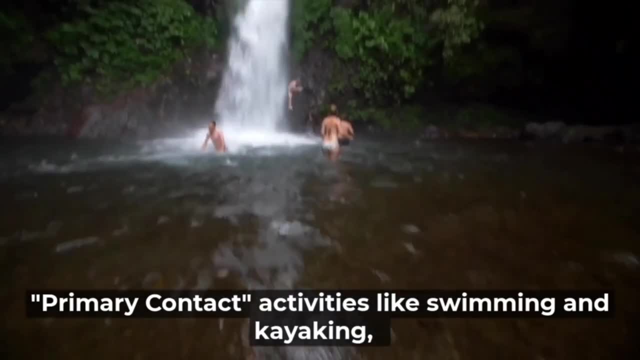 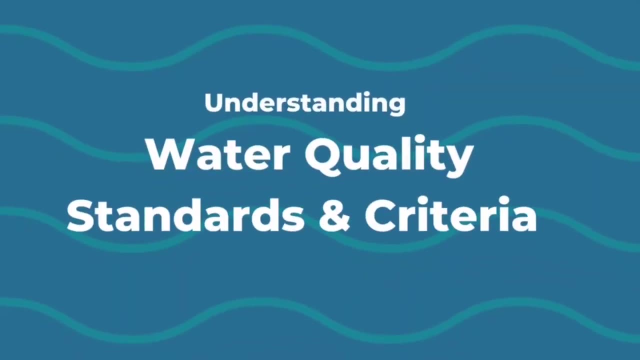 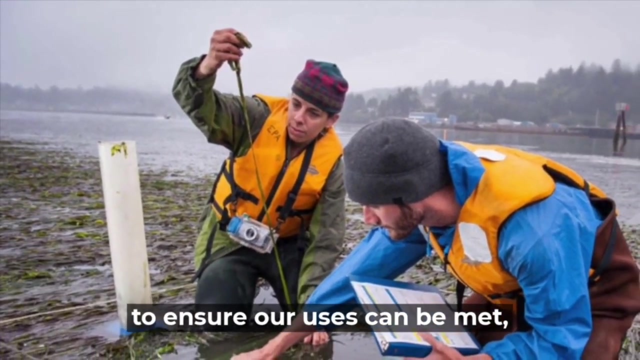 which includes activities like boating, where the chance of ingesting water is fairly low. Others are designated for primary contact activities like swimming and kayaking, for which waters need to be held to a cleaner standard. Water quality standards include different criteria to ensure our uses can be met. 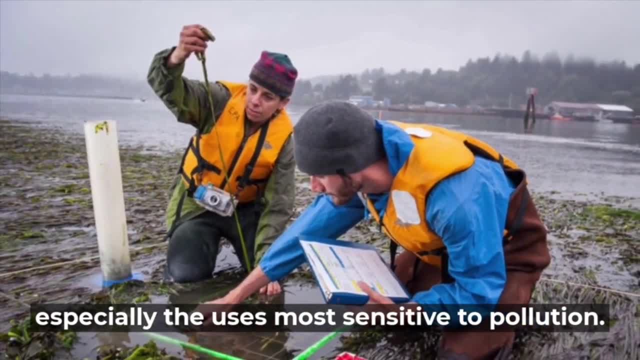 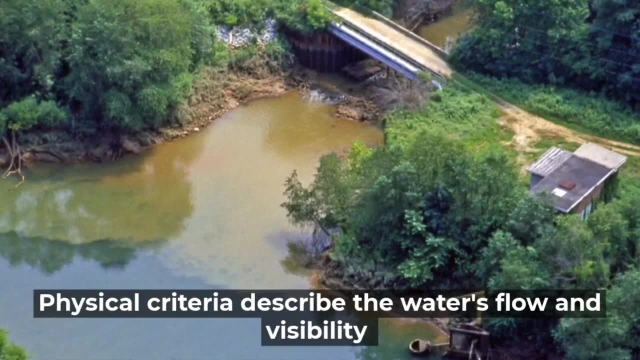 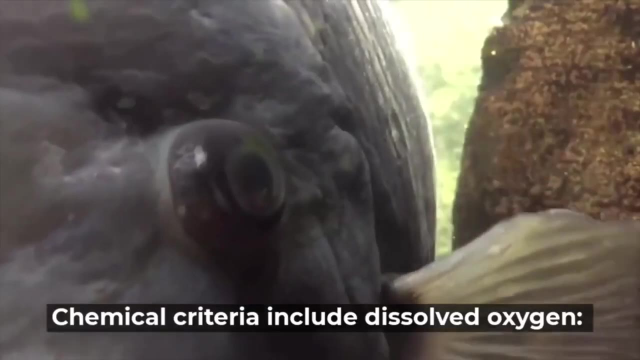 especially the uses most sensitive to pollution. Criteria can be physical, chemical or biological. Physical criteria describes the water's flow and visibility, and whether it's hampered by sediment and floating debris. Chemical criteria include dissolved oxygen: the level of oxygen available for aquatic life. 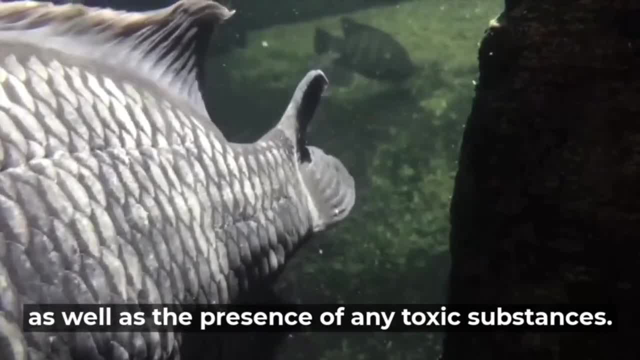 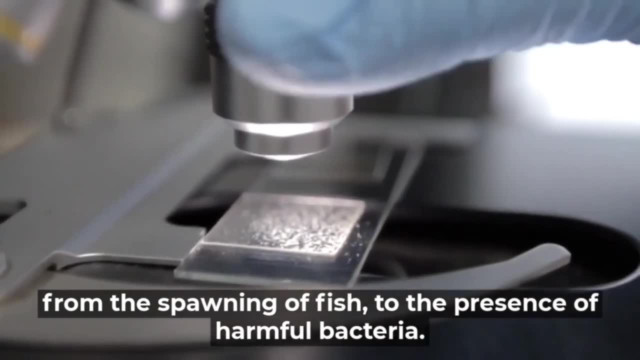 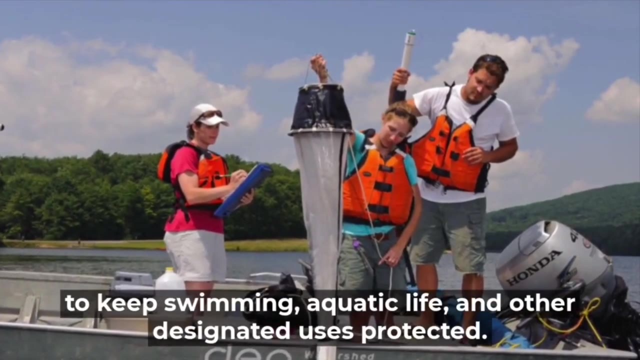 as well as the presence of any toxic substances. Finally, biology describes the balance of life in the water, from the spawning of fish to the presence of harmful bacteria. States are charged with monitoring all of these factors regularly to keep swimming, aquatic life and other designated uses protected. 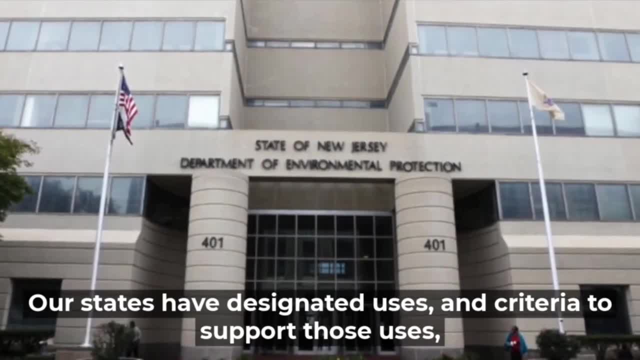 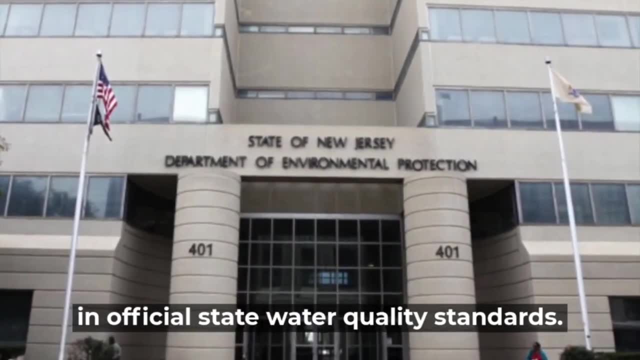 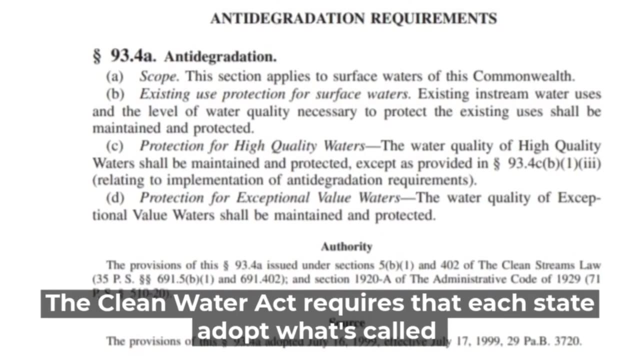 Our states have designated uses and criteria to support those uses, which the EPA has approved for inclusion in official water quality standards. So how do we achieve and enforce those standards? The Clean Water Act requires that each state adopt what's called an anti-degradation plan. 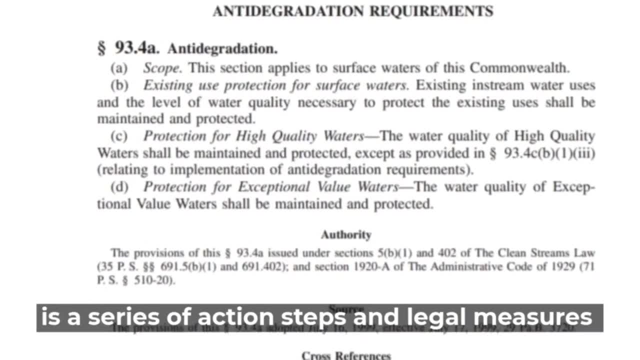 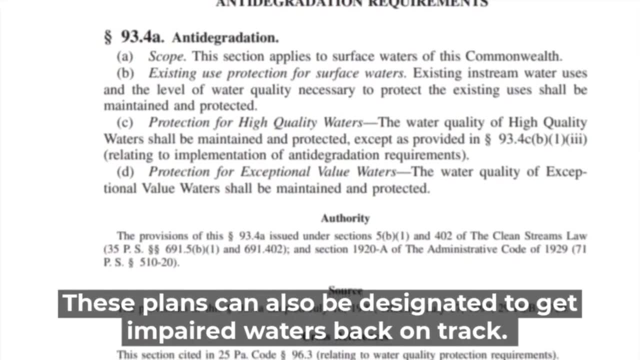 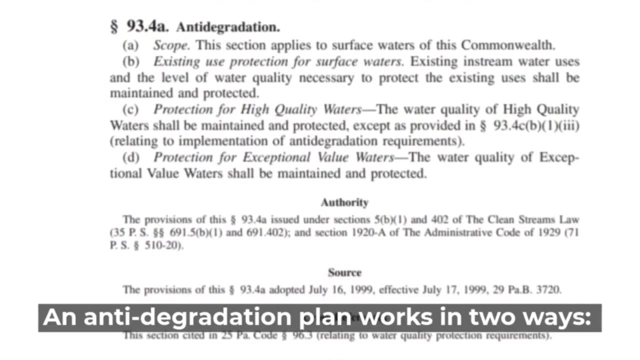 An anti-degradation plan, put simply, is a series of action steps and legal measures designated to keep healthy waters thriving. These plans can also be designated to get impaired waters back on track. An anti-degradation plan works in two ways: Through pollution permits that limit both the number of pollution sources. 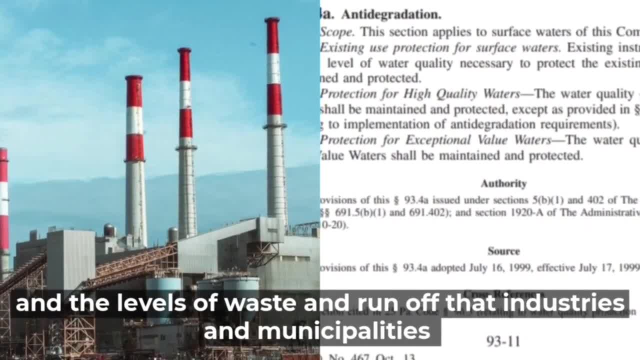 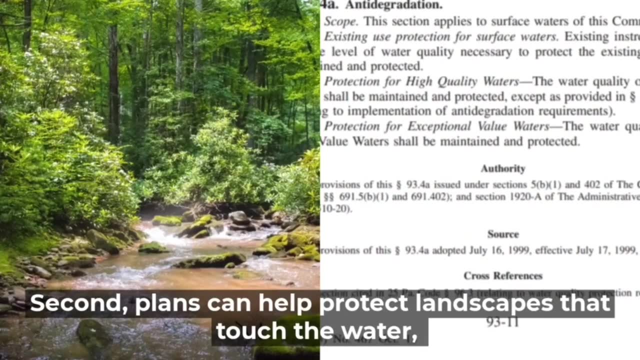 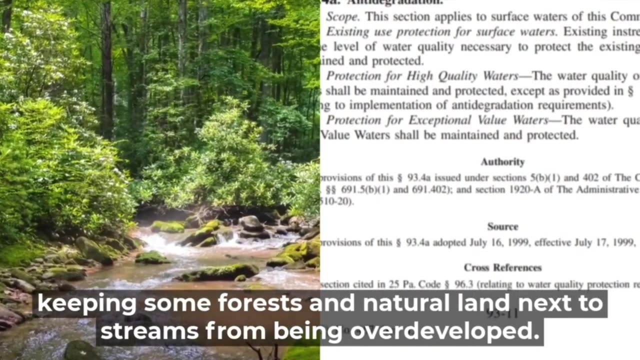 and the levels of waste and runoff that industries and municipalities are allowed to release into our waterways. Second plans can help protect landscapes that touch the water, keeping some forests and natural land next to streams from being overdeveloped, Even with standards, permits and plans in place.